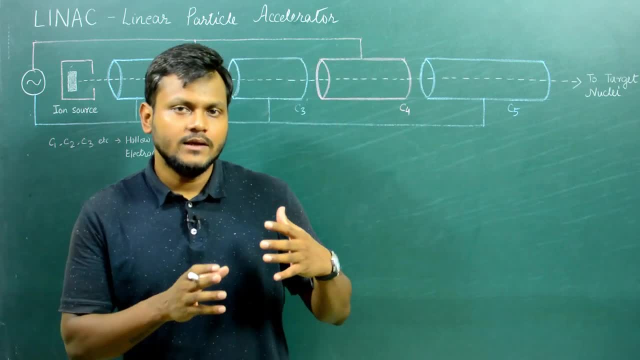 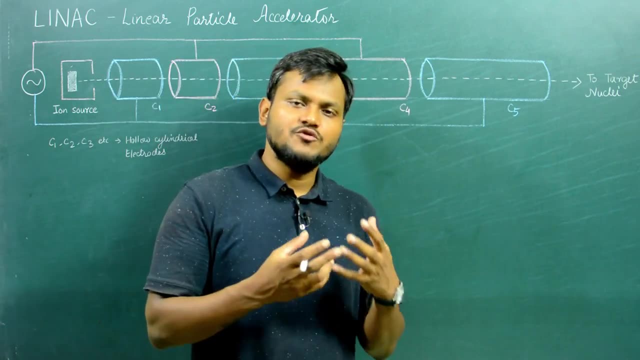 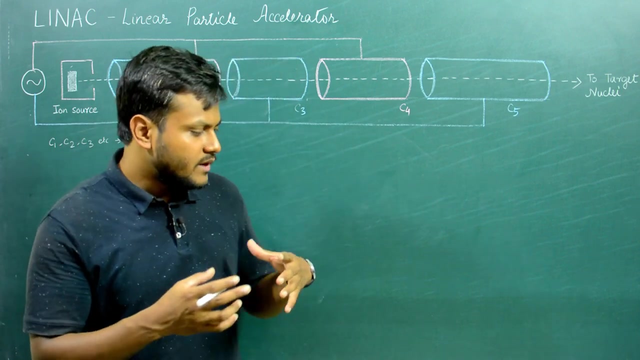 Hi. so in today's video I want to talk about the linear particle accelerator, or line app. So it's a special kind of an accelerator that can accelerate charged particles to very, very high velocities, so that those charged particles then can be used for suitable nuclear experiments. Now in my earlier 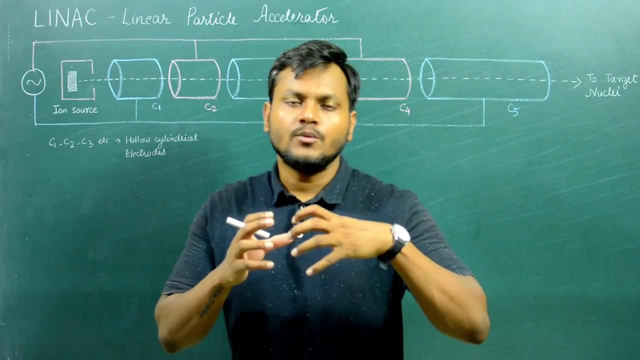 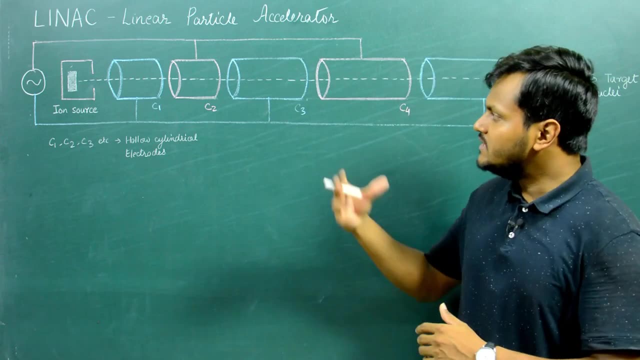 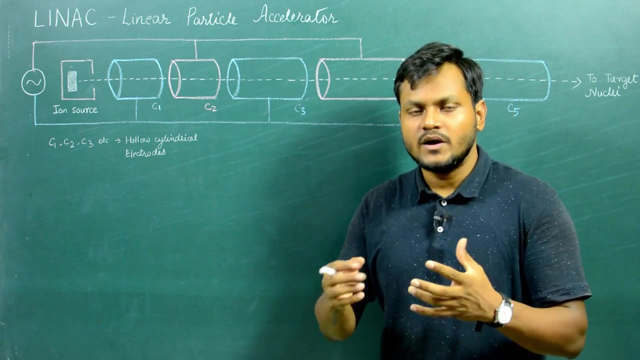 videos. I talked about the electrostatic accelerators. So, as opposed to electrostatic accelerators, this is an electromagnetic accelerator. So what is an electromagnetic accelerator? So in these kind of accelerators, a charged particle is accelerated by a potential difference by making the charged particle travel through the potential difference over and over. 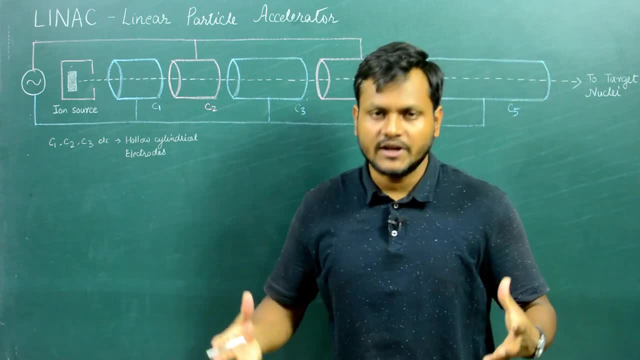 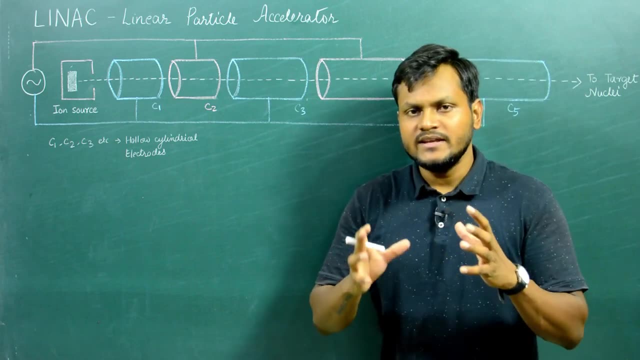 and over again by using some kind of alternating potential difference. So those kind of accelerators are known as electromagnetic accelerators, and line app is one of them. So I'm going to explain in detail what that actually means. So in this video I'm going to talk about the principle. 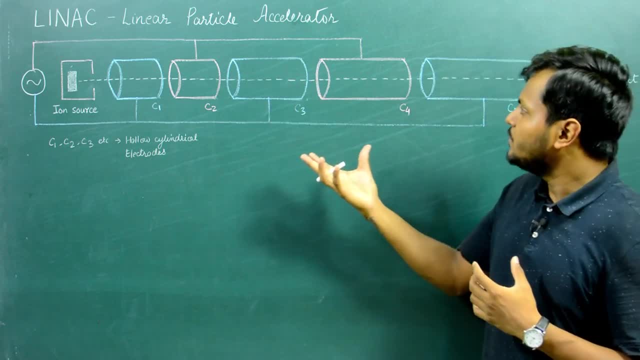 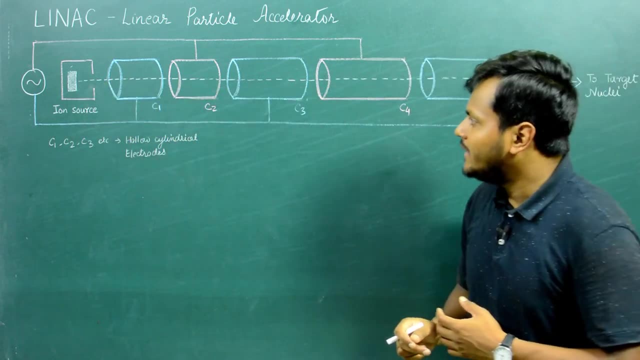 the construction and the working mechanism with which this kind of a linear particle is made. So what kind of Particle Accelerator works? It's called linear because a particle is accelerated in a linear fashion, in a straight line. So let's first talk about the construction. 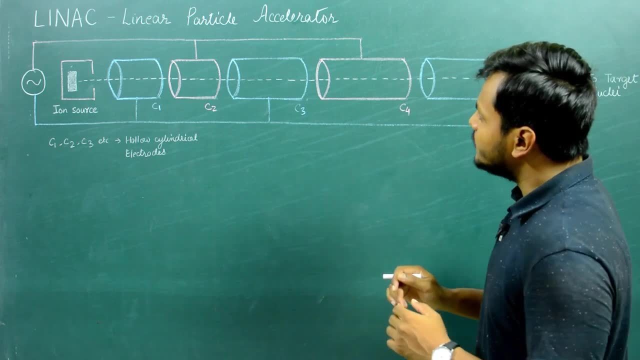 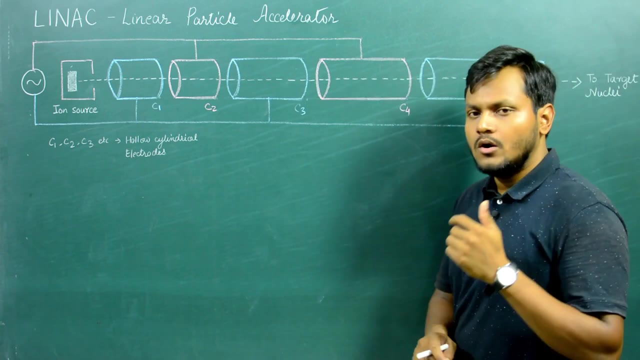 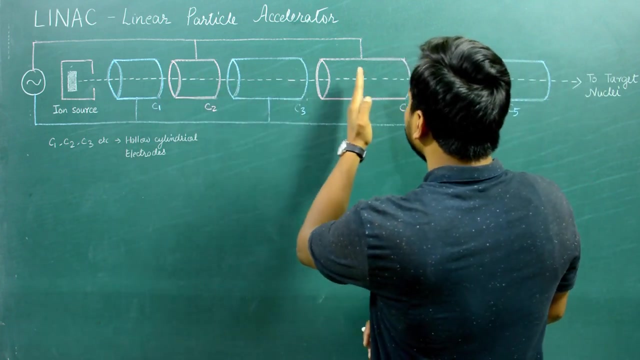 of this kind of a set up. So, as you can see here, the construction of this linear particle accelerator is composed of many number of cylindrical tubes. So these are metallic hollow open-ended cylinders or electrodes which are placed linearly in this kind of a fashion. 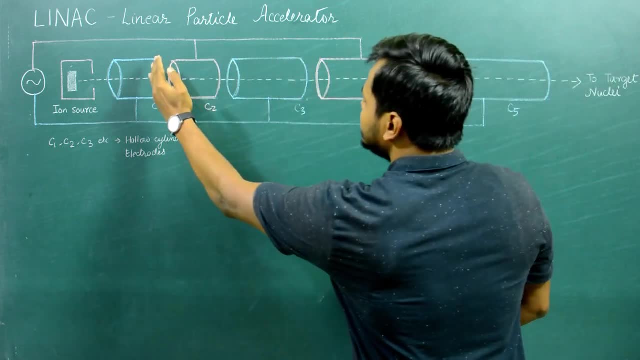 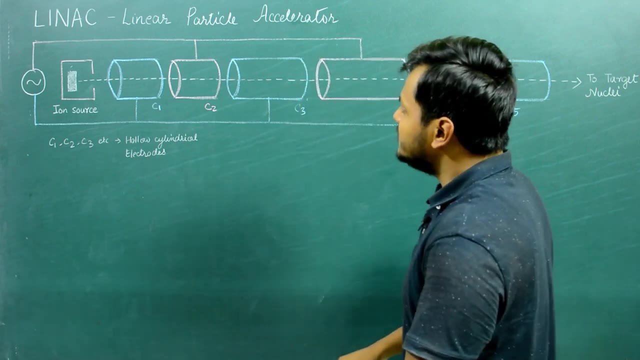 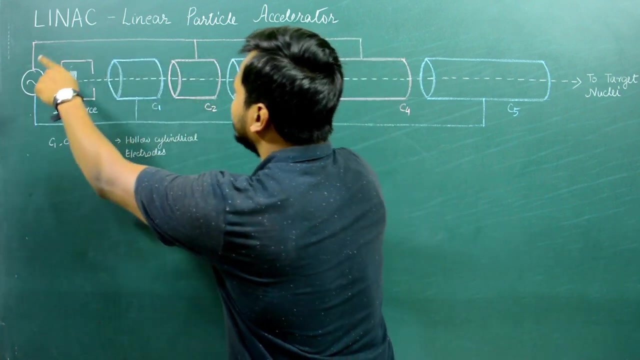 not each other. and every cylinder, alternatively, is connected to the opposite polarity of an AC supply here. so, as you can see here, every other alternate cylinder is connected to the opposite polarity. every other cylinder is connected to the opposite polarity of some kind of a alternating potential difference. now how does that help? we'll understand this. 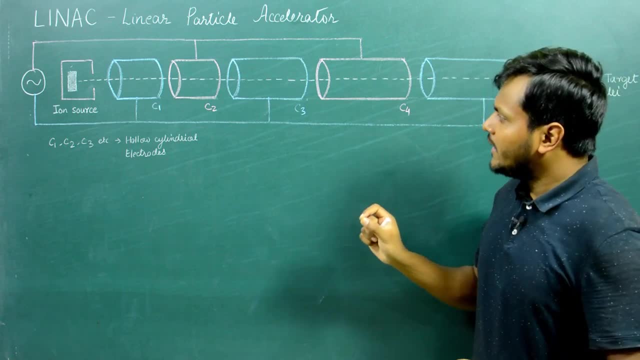 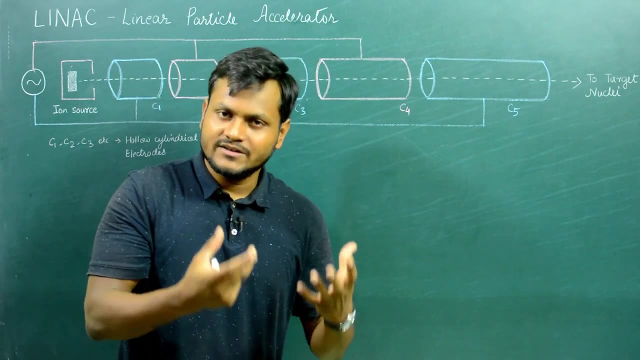 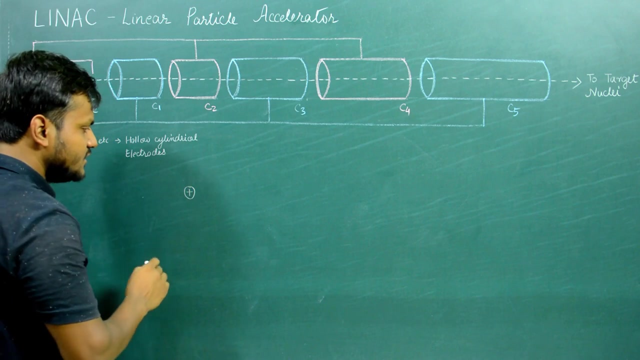 when you look at the working mechanism. so before you talk about the working mechanism, let's understand the principle here. the principle is very simple: if a charged particle is present in a region where there's an electric field, then it will get accelerated. so, for example, if you have a charged particle, let's suppose it's positively charged and I name this as. 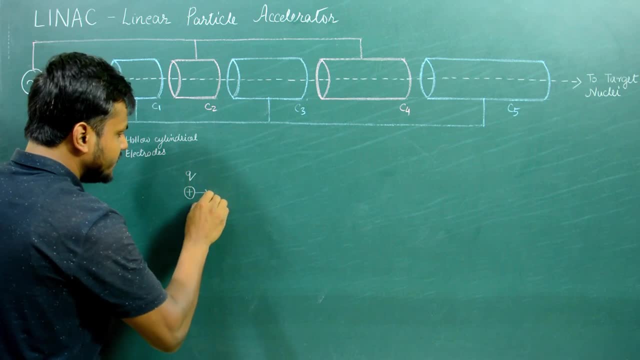 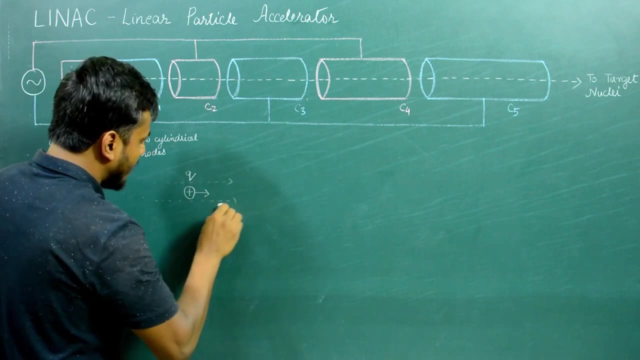 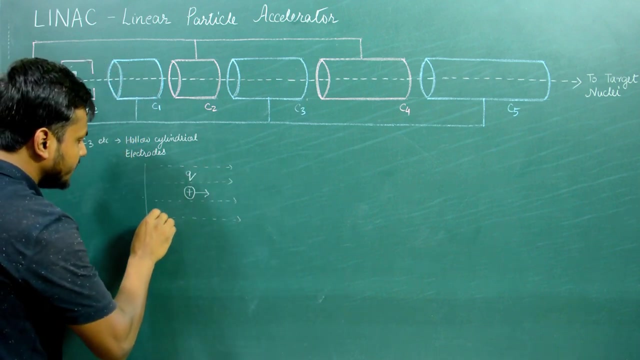 Q- if this kind of a charged particle is moving in a certain direction and I place it in the presence of some kind of a external electric field? so how do I create an external electric field? Well, we can create the external electric field by placing this charged particle in. 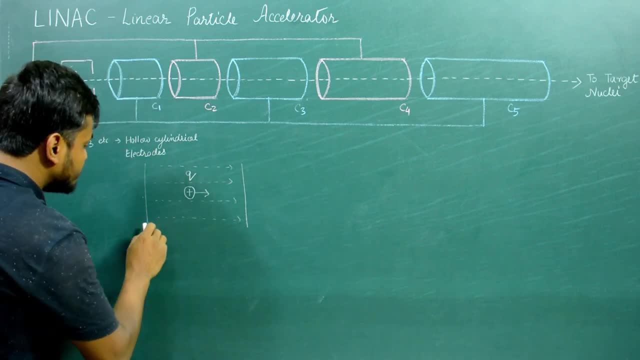 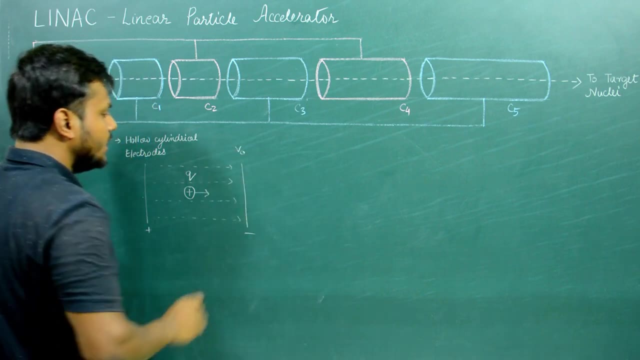 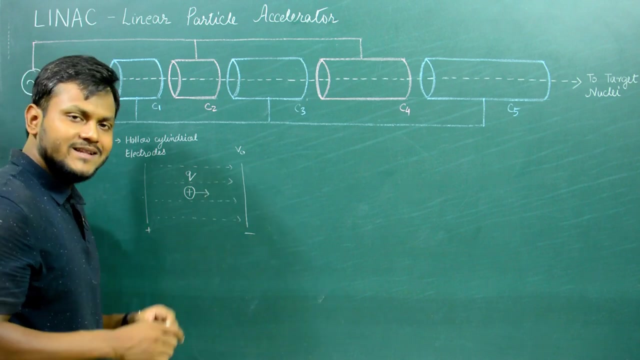 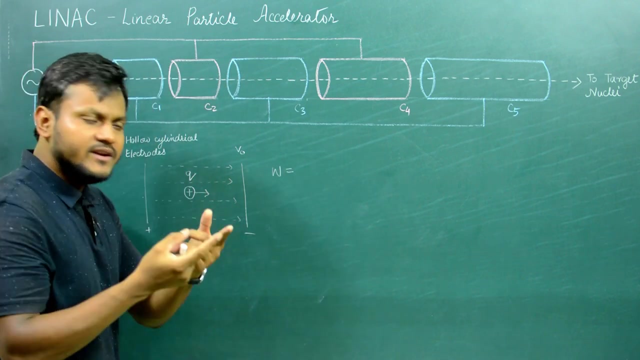 between two electrodes or terminals which are at different potentials. let's suppose the potential difference between these two terminals is given by V naught. now if a charged particle, Q, is present in between a potential difference or v naught, then the total amount of work done, the total amount of work done in increasing the kinetic energy of the charged. 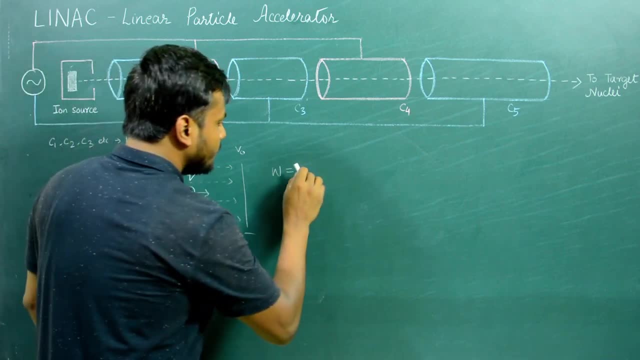 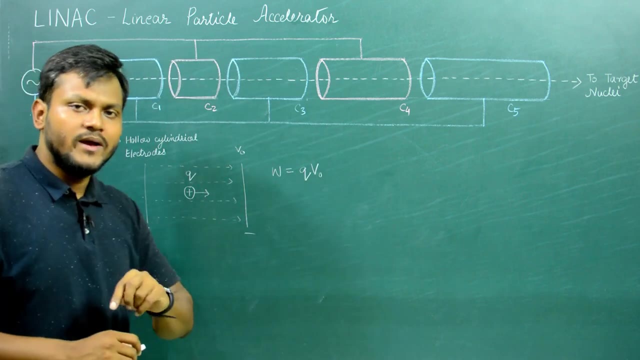 particle is given to the existing terminal. If a charged particle Q is given to a potential particle as it moves from here to here, is basically given by the charge of the charged particle multiplied by the potential difference. so this is something that I proved in one of my earlier videos. so the total amount of 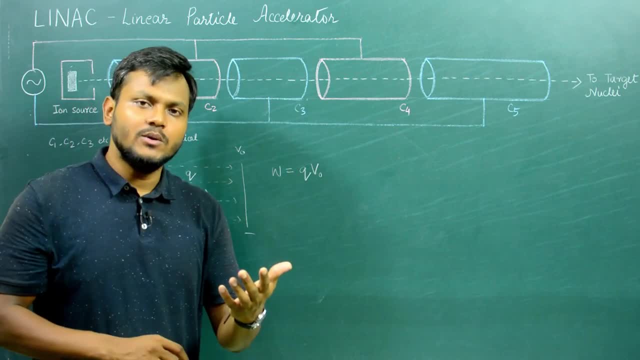 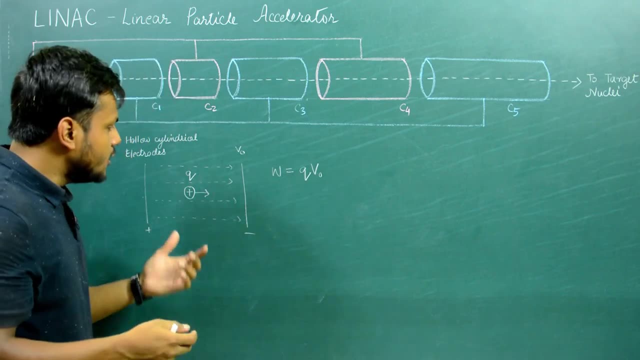 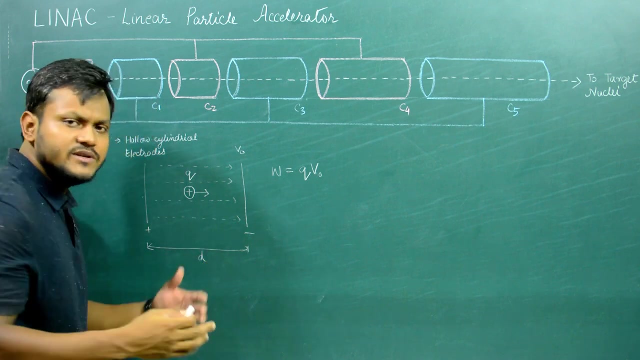 work done, or the increase in kinetic energy is basically equal to the charge multiplied by the potential difference. now, what is work done? work, then, is nothing but force multiplied by distance. so let's suppose that this distance is nothing but some D centimeters or something like that. so force multiplied. 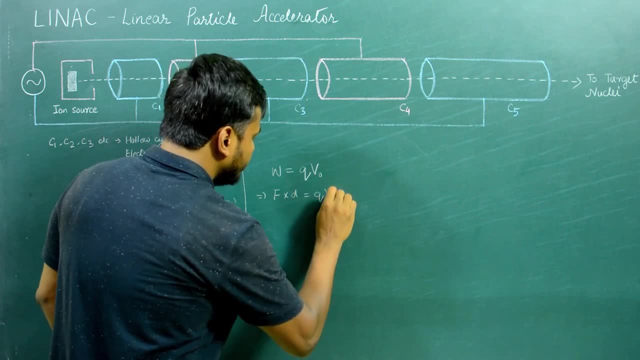 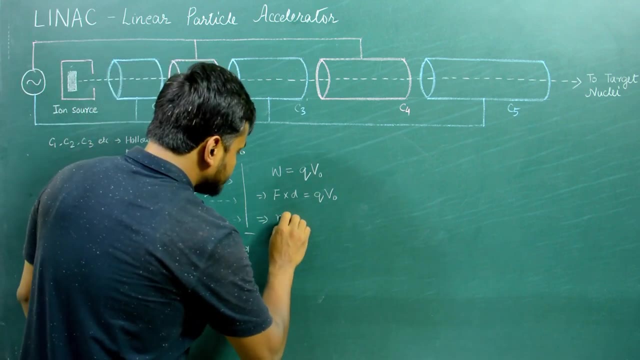 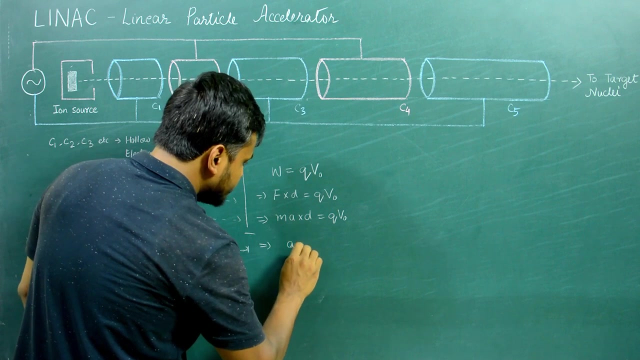 by distance is Q V naught. what is force? this is force is because of the electric field, but I can write this here as mass times acceleration. so mass times acceleration multiplied by the distance is equal to Q V naught. or the acceleration is equal to Q V naught upon MD. so the acceleration 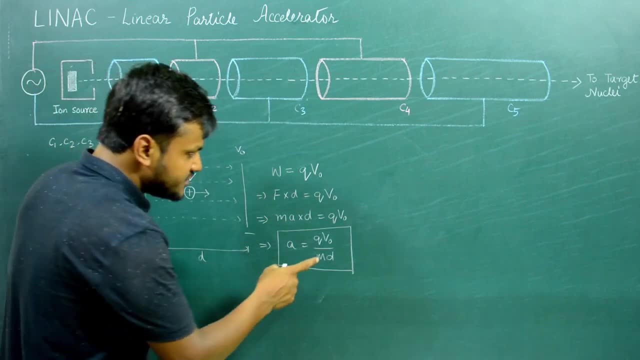 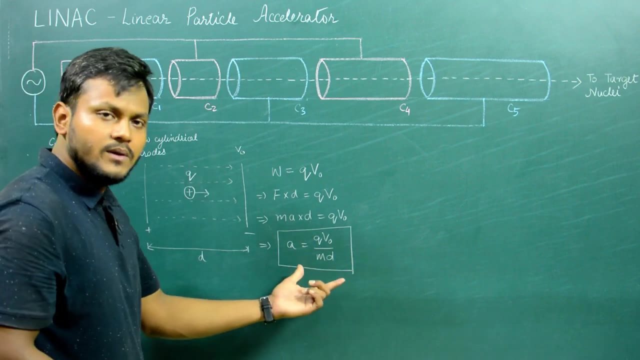 experienced, Experienced by the charged particle because of a potential difference V0,. having mass m and charge q along a distance of d is basically given by this Quite simple right. So the greater the amount of potential difference V0,, the greater is going to be the acceleration. 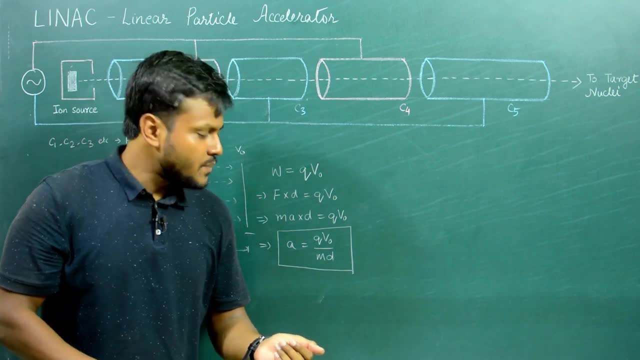 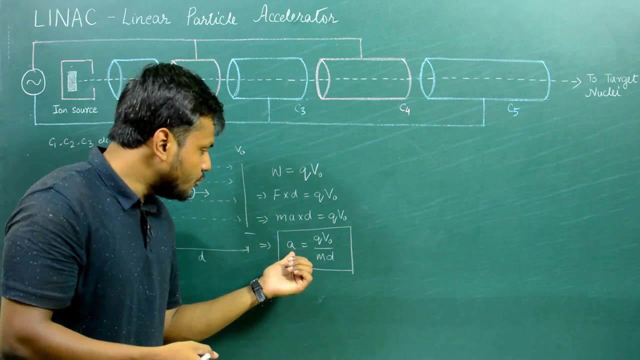 Now in one of my previous videos where I discussed Van de Graaff's generator, there is a huge amount of potential difference that is created and the charged particle experiences a huge amount of acceleration proportional to the potential difference. However, in electromagnetic accelerators, the potential difference is not very high. 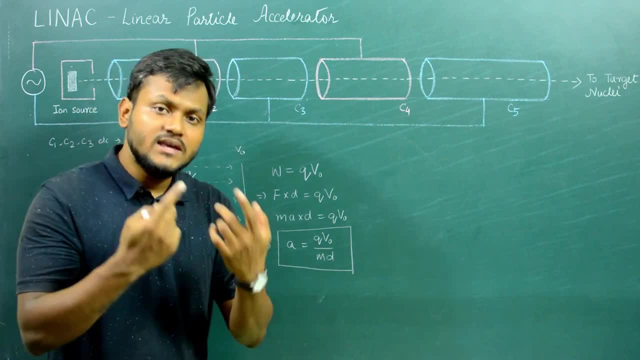 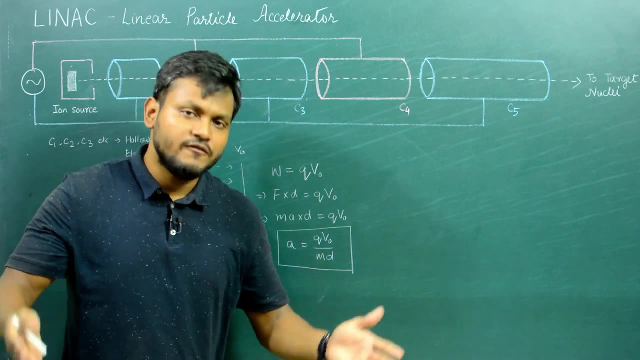 But we can achieve huge accelerations by making the charged particle accelerate because of that potential difference over and, over and over again, many number of times. Now how that is done can be understood by looking at the working mechanism in this kind of a setup. 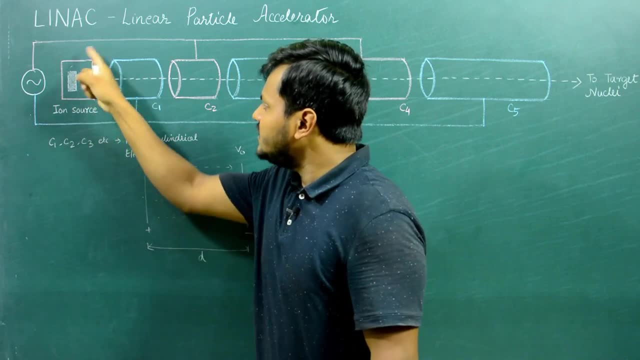 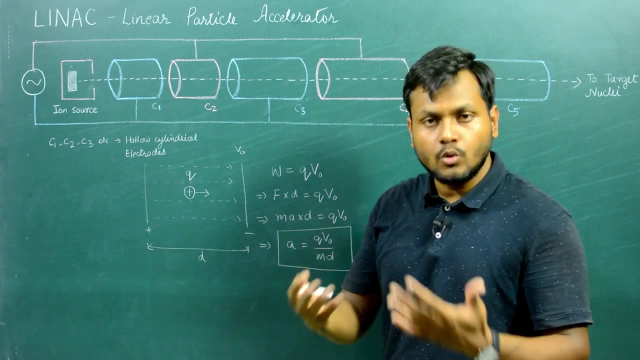 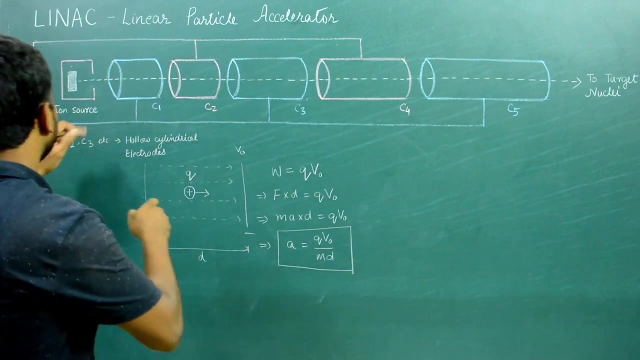 So here the first cylinder. this cylinder you can see here contains some kind of an ion source. So ion source is some kind of a source That emits radioactive particles, let's suppose like protons or alpha particles. Now let's suppose that the moment a charged particle is emitted from this ion source. 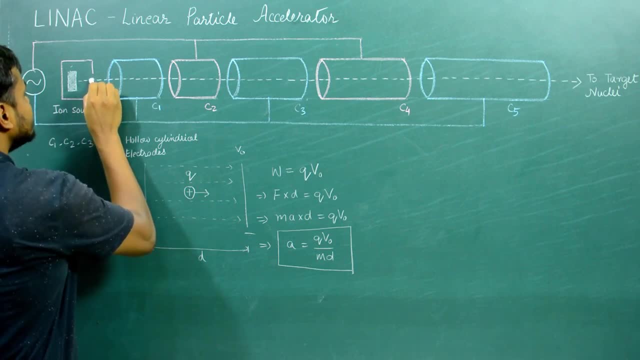 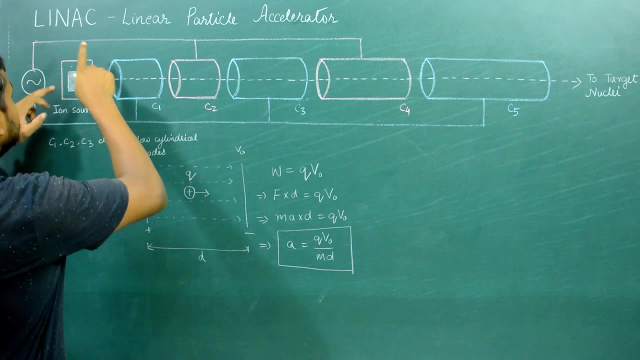 all right, let's suppose there is charged particle. Let's suppose that this is a positive charged particle. all right, The moment the charged particle is emitted from the ion source, then the nature of the alternating potential is such that this is at a positive terminal. 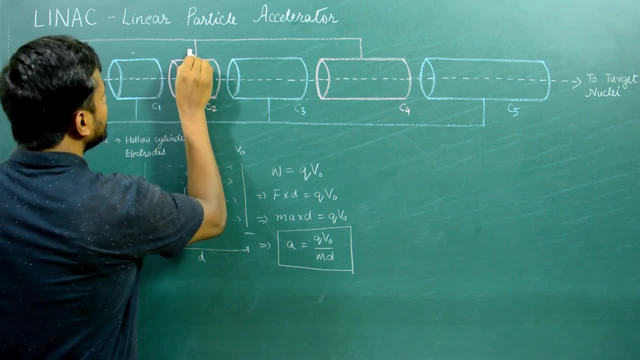 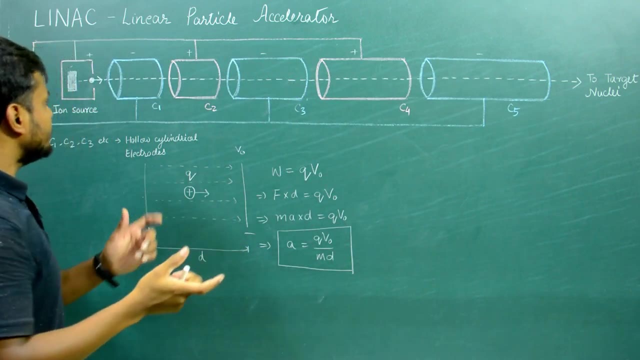 Let's connect these two. This is at a negative terminal, This is at a positive terminal, This is at a negative terminal, This is at a positive terminal and this is at a negative terminal. So, because of this, what happens is that in these gaps between these cylinders, there 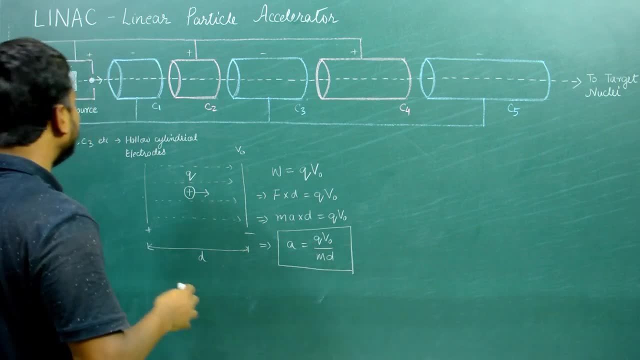 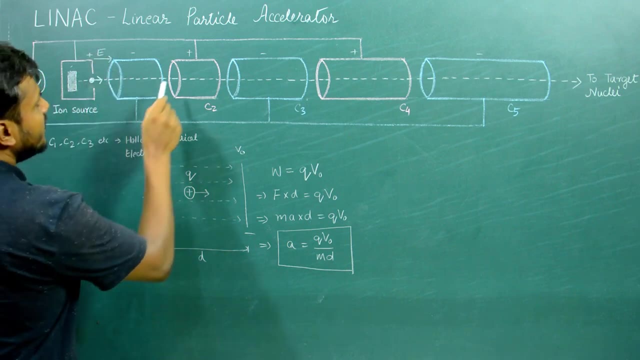 is going to be a potential difference which is going to create an electric field. So, for example, because this is positive and this is negative, there is going to be an electric field in this direction. In this case, the electric field is going to be in the opposite direction. 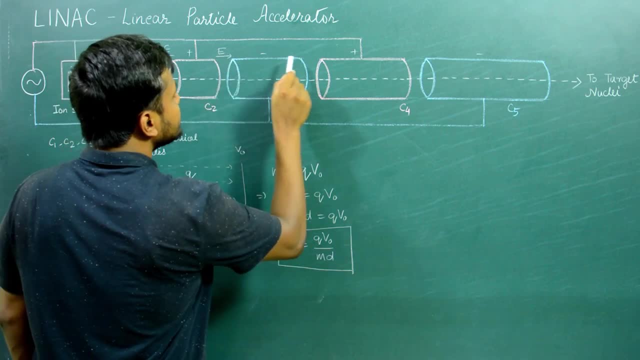 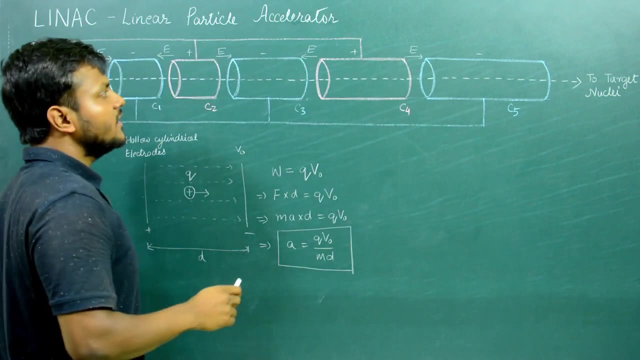 In this case, the electric field is going to be in this direction. In this case, the electric field is going to be in the opposite direction. In this case, the electric field is going to be in this particular direction, right. So now, the moment this charged particle- which is positive, let's suppose- like an 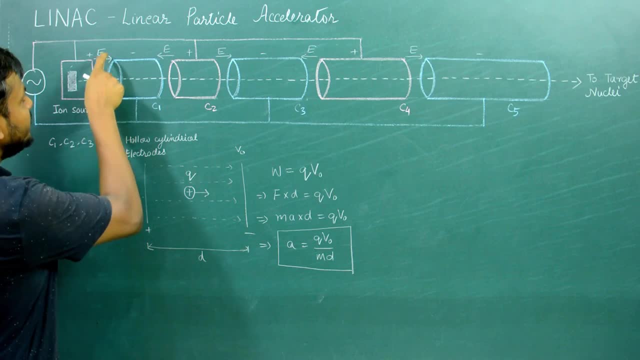 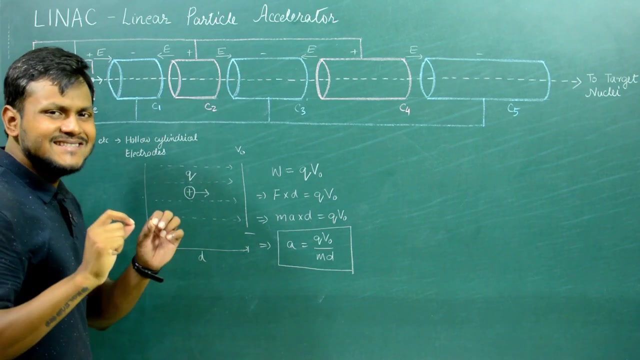 alpha particle is emitted in this gap, it experiences an electric field of E. all right, This electric field of E is basically a result of the potential difference V0 between this and this. So because of this positive electric field in this direction, it gets associated. 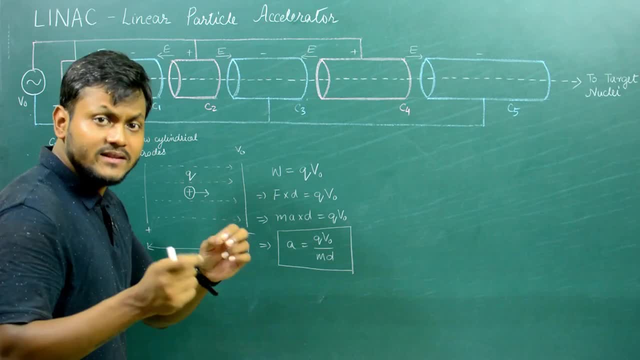 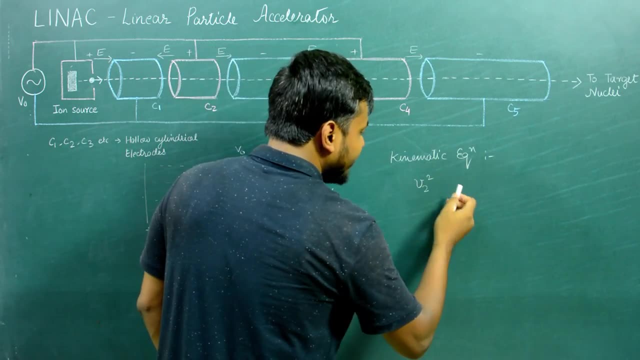 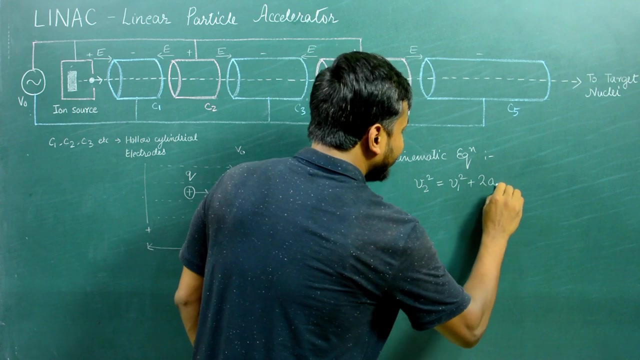 It gets accelerated by this particular amount. We can calculate the increase in velocity by using the kinematic equations. So, for example, we know that the final velocity is basically equal to V2, where V2 square is equal to V1 square plus 2AD, where D is the distance between these two cylinders. 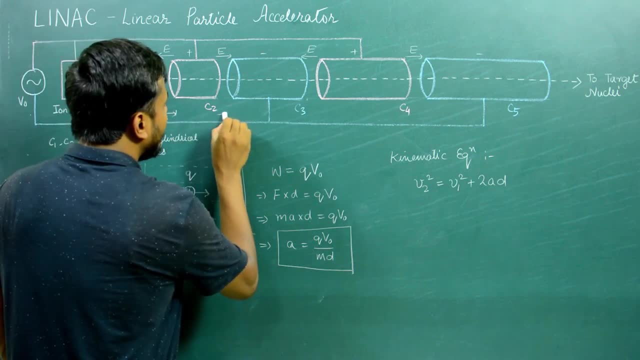 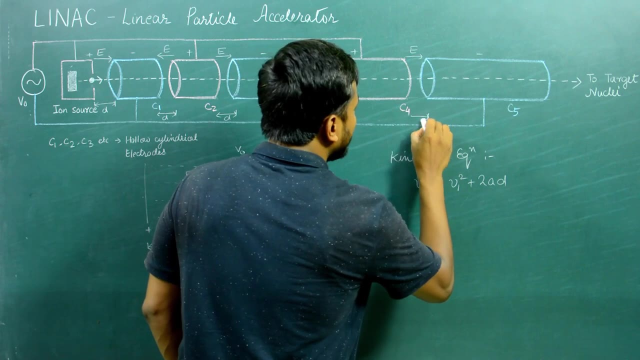 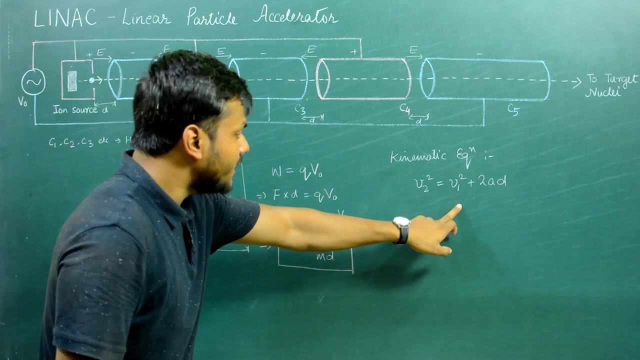 Let's suppose every single cylinder is separated by a distance of D. all right, So every single cylinder is separated by a distance of D. So let's suppose the moment ion source emits an ion particle, it has a velocity V1.. 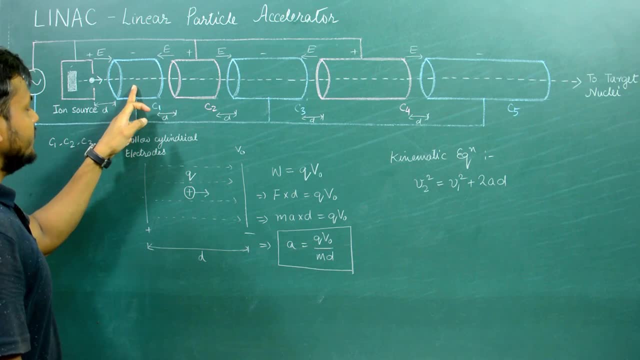 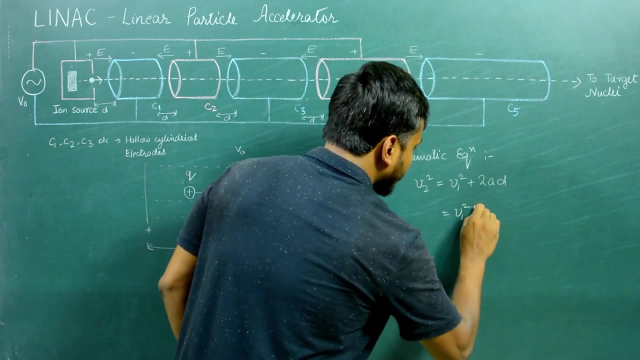 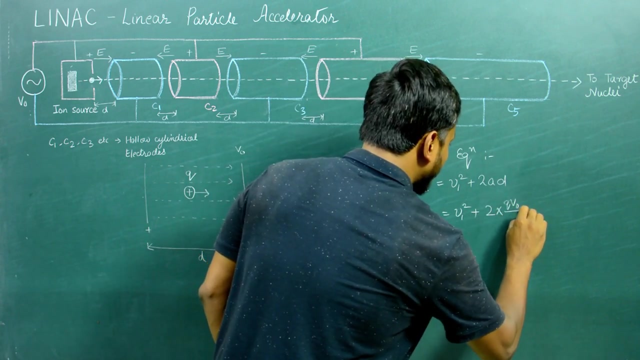 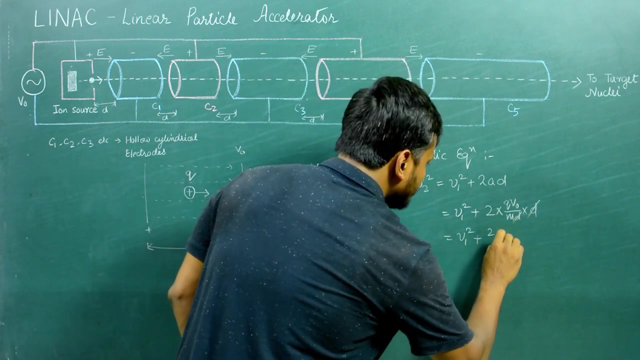 Then, as it gets accelerated in this region before entering the cylinder C1, its velocity basically becomes V1 square plus acceleration. A is so 2 multiplied by QV0 upon MD. So as you can see here, something very interesting. 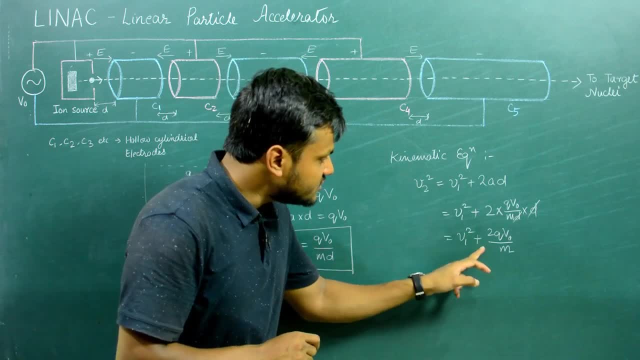 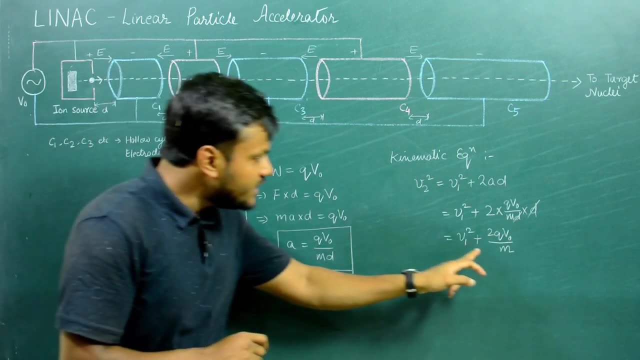 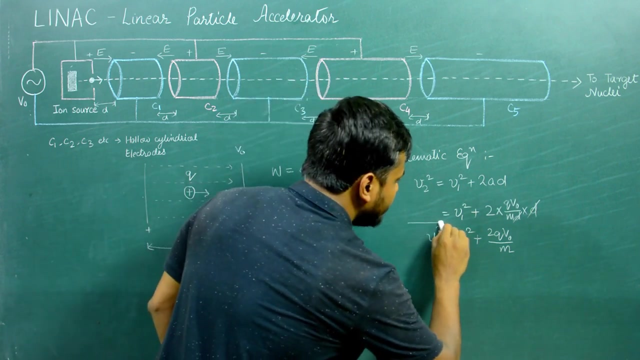 The increase in the velocity. the change in the velocity is not dependent upon the distance, It does not depend upon the separation distance between these cylinders. It only depends upon the potential difference V0.. So the final velocity, V2 square which is greater than V1 square is basically dependent. 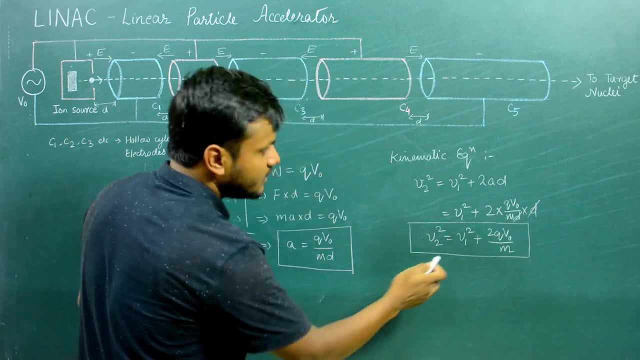 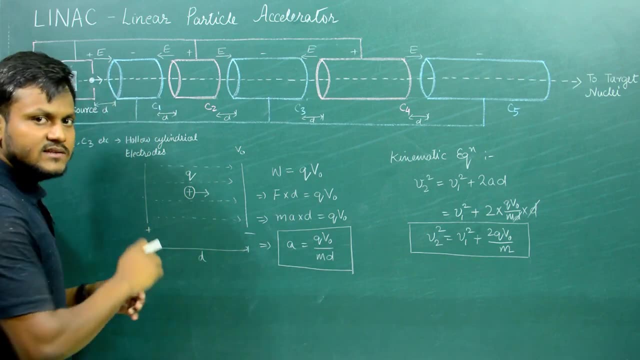 only on the potential difference and the mass and the charge of the particle. So using this equation we can calculate the increase in the velocity. Now, once it gets accelerated, it enters the second cylinder. Now, inside the cylinder the potential is constant, The potential difference. 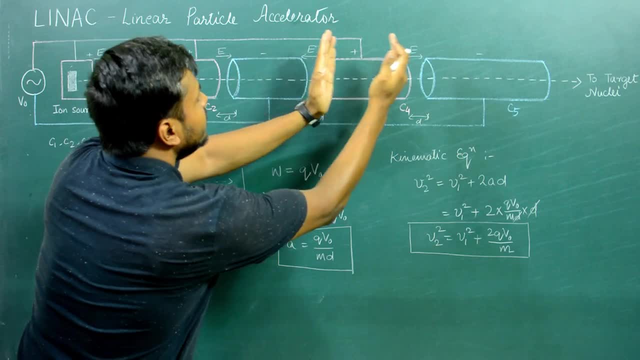 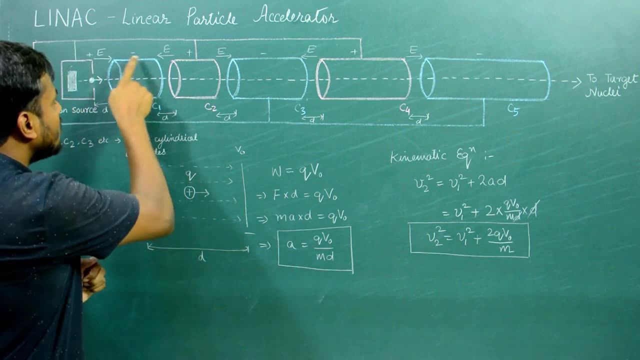 only exists in these separation regions between these alternate cylinders, But inside the region, in the cylinder, the potential difference is zero because it is at a constant potential, Whether it is negative or whether it is positive, it is at a constant potential And in a region of constant. 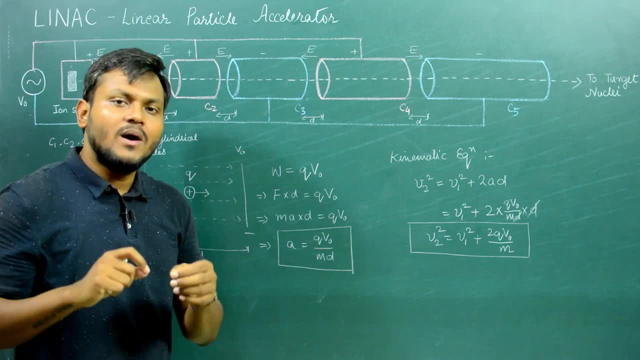 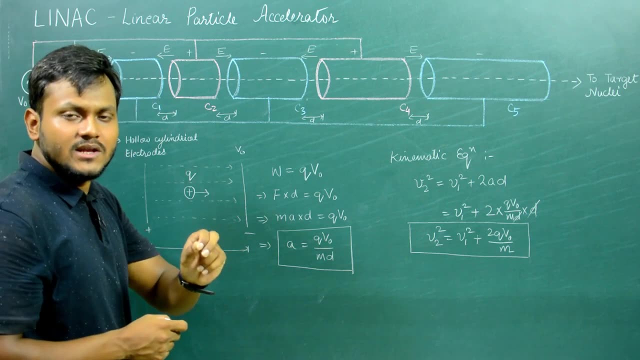 potential, there is no electric field. And if there is no electric field the particle does not get accelerated. So the moment the particle enters a cylinder it enters a region of constant potential And because of this there is no acceleration anymore. It travels at that fixed. 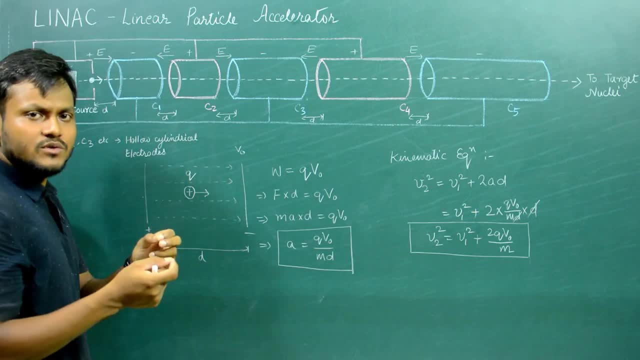 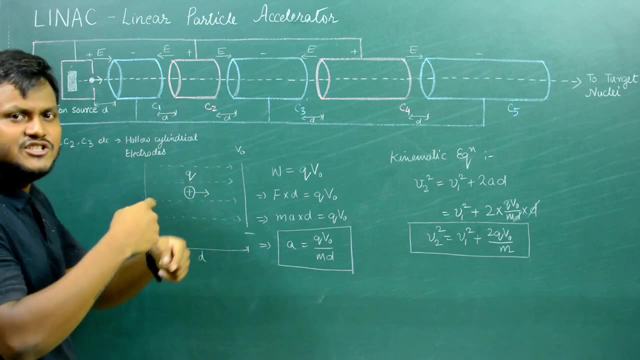 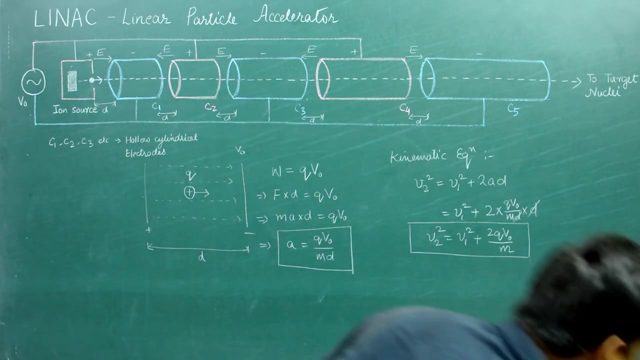 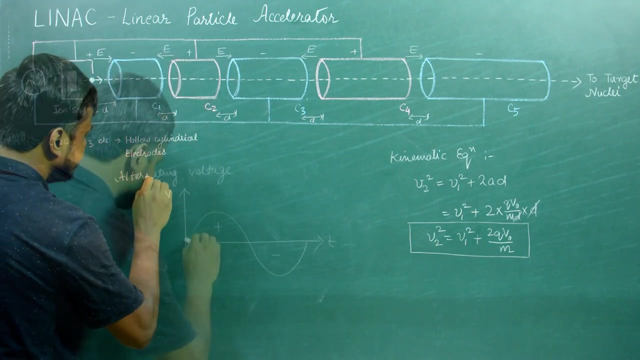 velocity throughout that particular cylinder. Now let's suppose that the moment it is about to exit the cylinder, the polarity of this signal suddenly changes. So basically, this is an alternating voltage whose polarity is constantly changing. So let's rub this first. So the alternating voltage has maybe- let's suppose- this kind of a signal. 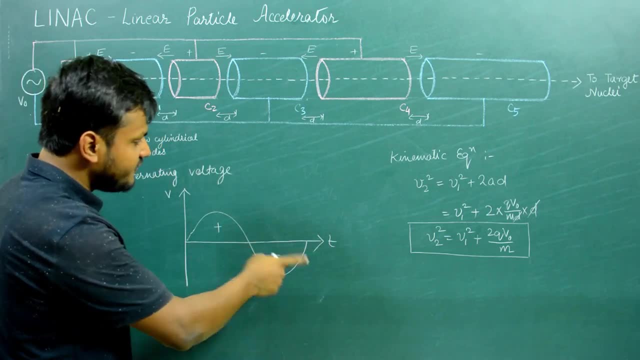 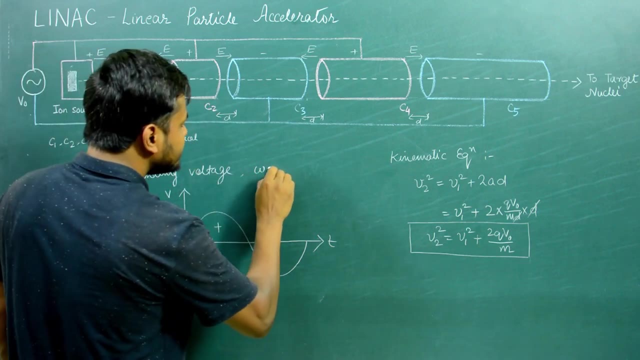 So voltage gets alternated between positive and negative over a period of time. So let's suppose the frequency of this kind of a signal is given by omega. So what is omega? Omega is nothing but 2 pi upon capital T, where the T is the time period of one complete oscillation. 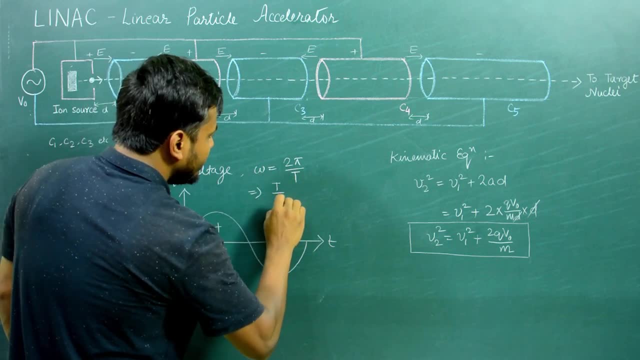 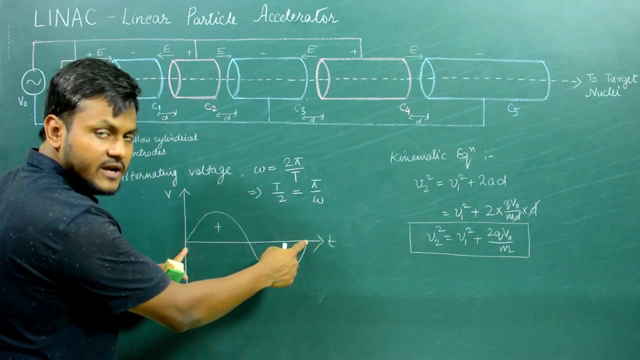 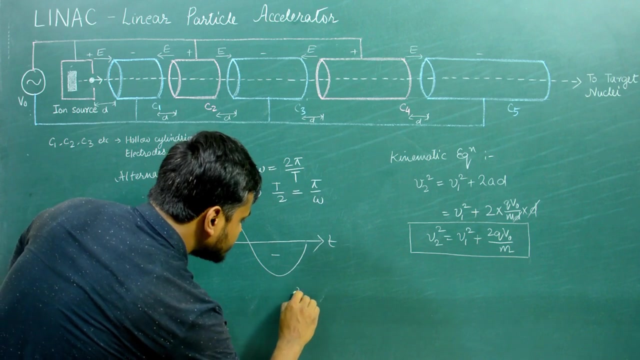 So I can write this as T upon 2 is basically equal to pi upon omega. Why I'm saying this is because T upon 2, T is the time period for complete oscillation, T upon 2 is the time period for one half of the cycle. So T upon 2, let's suppose, is written by small. 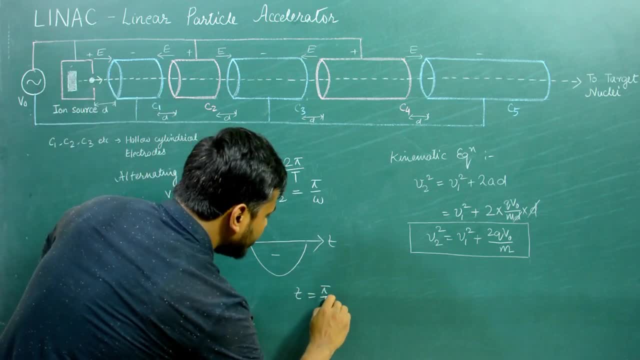 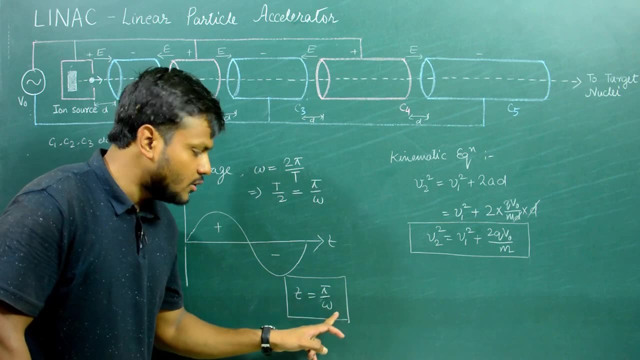 t. So one half of the cycle is basically equal to pi upon omega. So this is basically fixed based upon our construction. So one half of the cycle is equal to pi upon omega, where omega is the angular force. Thank you. 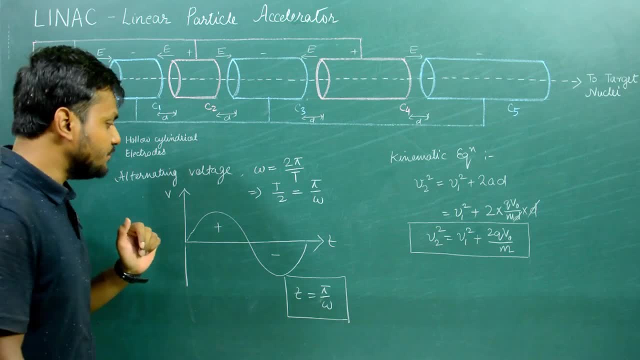 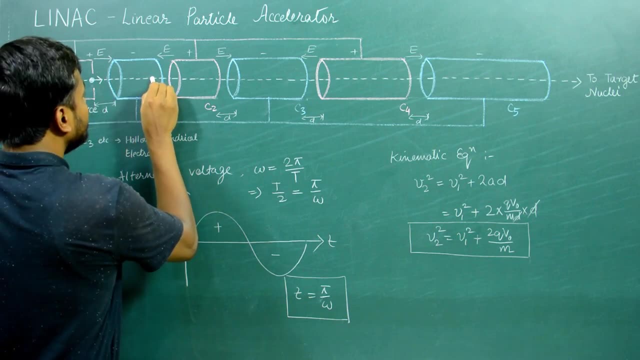 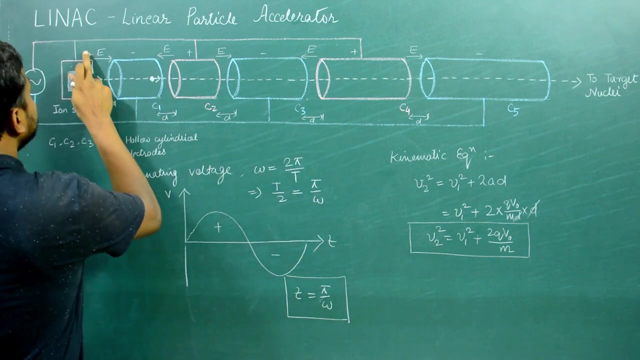 frequency of this kind of a radio source that we are using. So now, let's suppose that this is fixed in such a manner that once the charged particle reaches here, before it exits this cylinder, the polarity gets reversed again. So if the polarity gets reversed now, this becomes negative, this 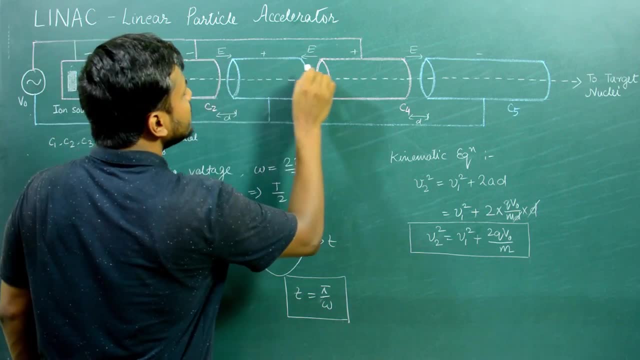 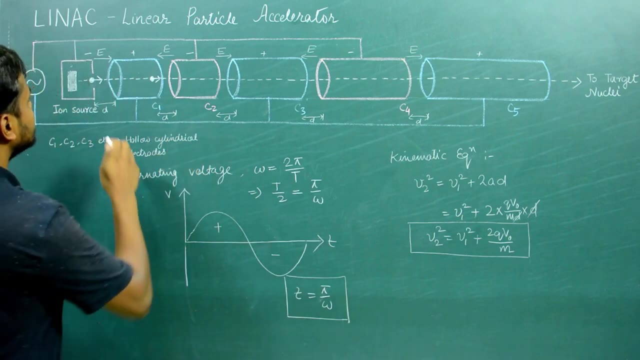 becomes positive, this becomes negative, this becomes positive, this becomes negative and this becomes positive. Now the electric field in between the cylinders also reverses in sign. So now this electric field is in this direction. this electric field is in the forward direction. 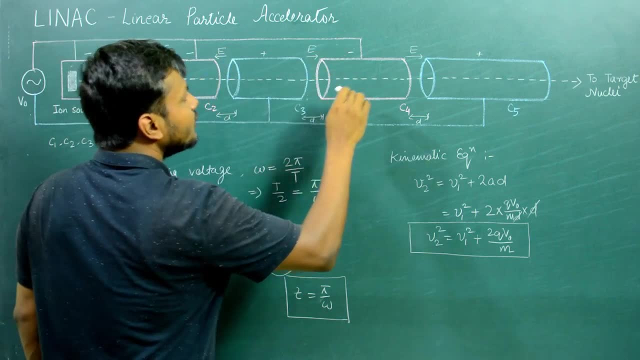 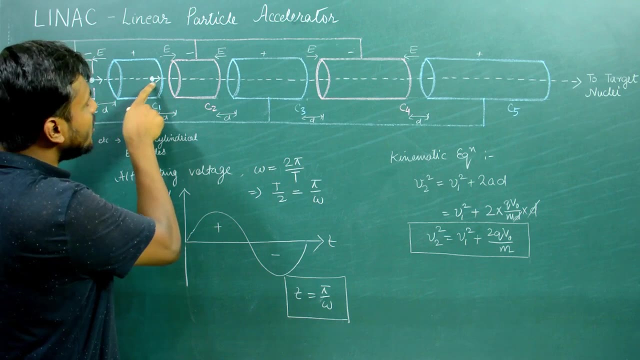 this electric field is in the reverse direction. this electric field is in the forward direction and this electric field is in the reverse direction. Now look at the interesting thing here. the charged particle is about to exit cylinder C1, but the electric field is facing in the forward. 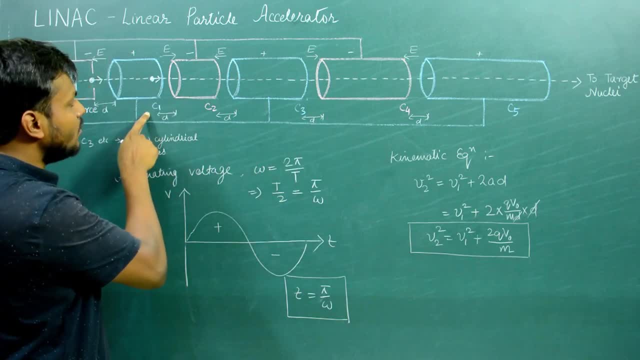 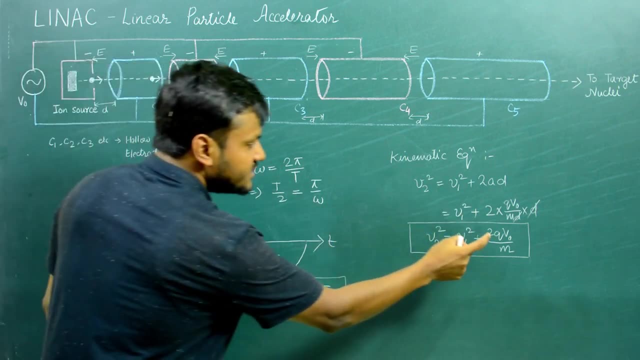 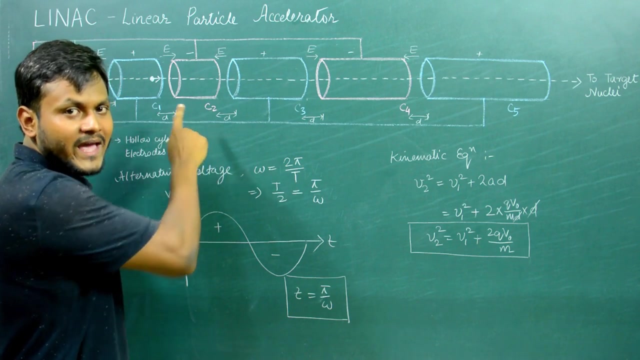 direction. That means once it exits the cylinder C1 and before it enters the forward direction and enters the cylinder C2 again, it will get accelerated in this particular region by the same amount. So again it gets accelerated and it enters the second cylinder, C2, and again the polarity. 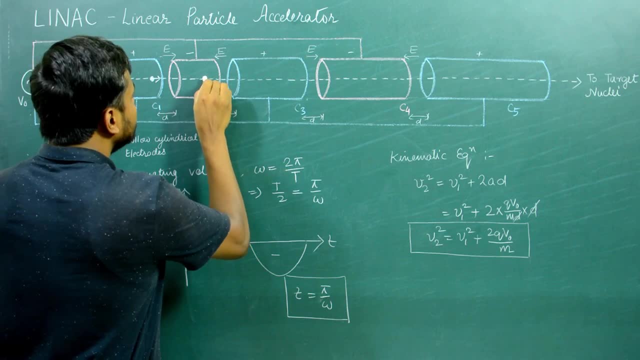 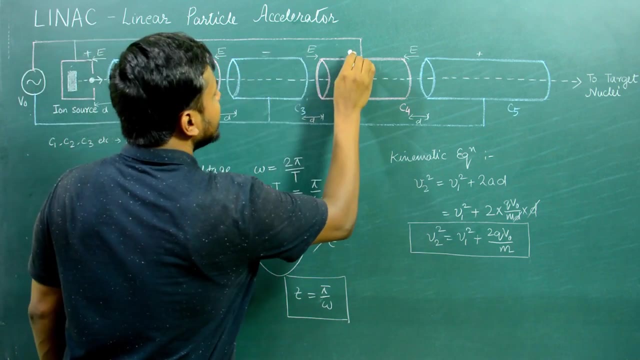 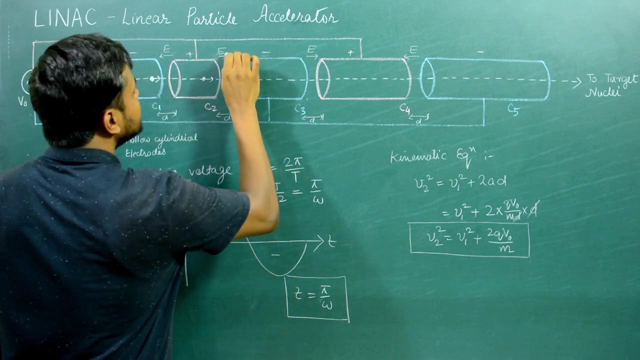 reverses. So once the charged particle comes here, the polarity again reverses, this becomes positive, this becomes negative, this becomes positive, this becomes negative, positive, negative here. So the electric fields also reverse in sign. this becomes reversed, this becomes forward, this becomes reversed and this becomes forward. 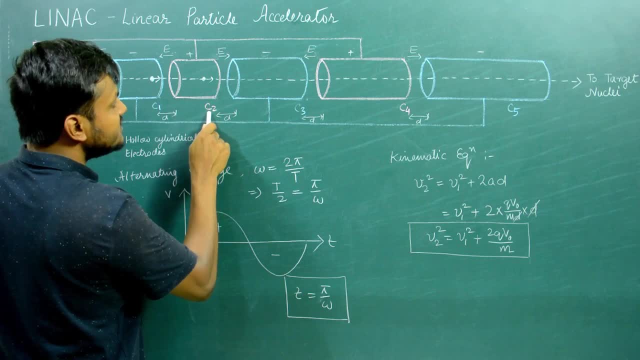 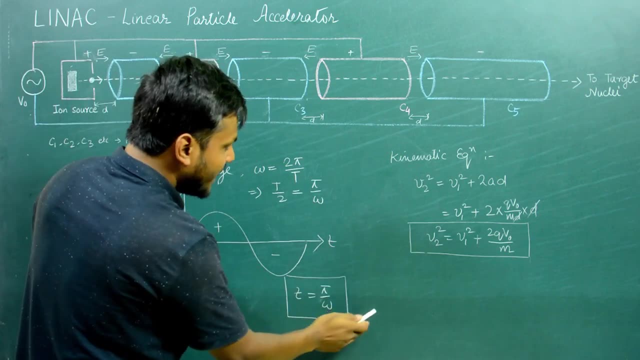 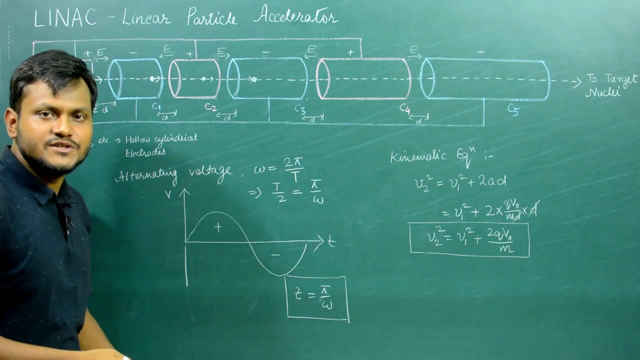 So now again, as the charged particle is about to exit C2 and enter C1, it experiences an electric field in the forward direction. So now again it gets accelerated by that particular amount. So again it enters the next cylinder and again the polarity reverses and as it exits it experiences: 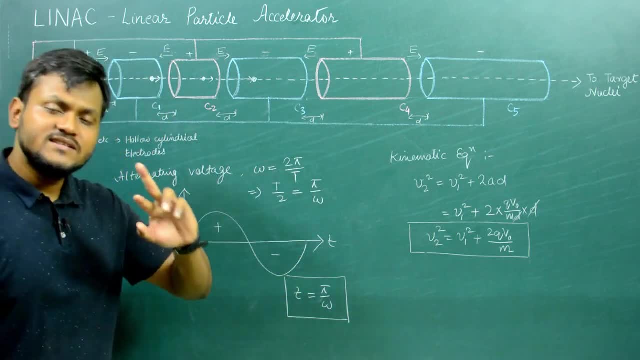 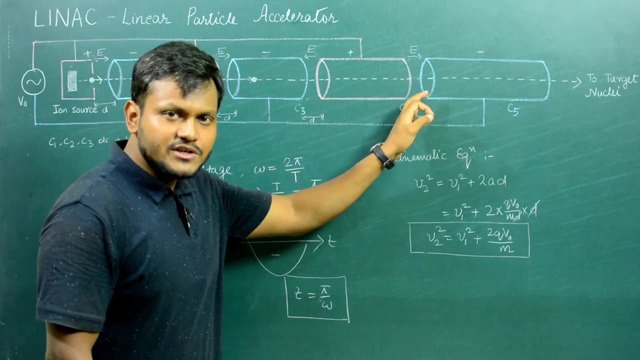 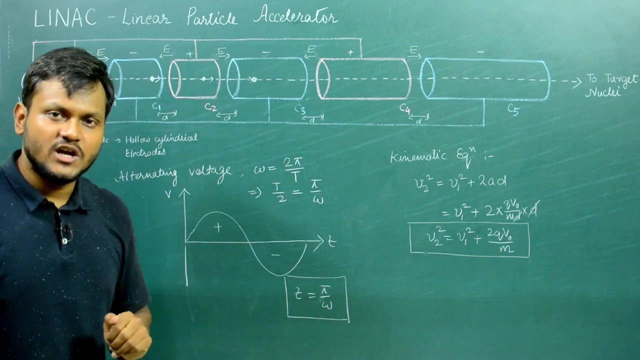 a positive electric field and again the polarity reverses, and this keeps happening over and over again, so that everytime the charged particle is in the intermediate region, it always experiences an electric field in the forward direction, so that the acceleration happens to the motion of the charged particle. So, to summarize, let's look at this particular animation here as the ion source. 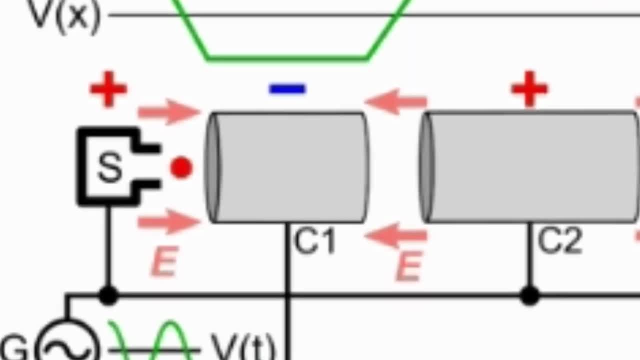 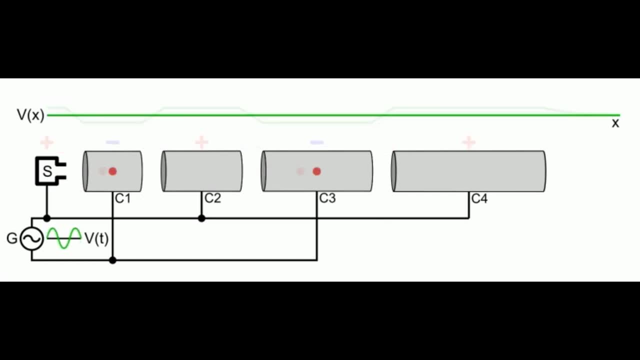 emits an ion particle, it experiences a positive electric field and it gets accelerated. The moment the charged particle enters the first cylinder the polarity gets reversed. Inside the cylinder it does not accelerate, but moves at constant velocity. but because the polarity gets reversed as it exits that first cylinder again, it experiences a 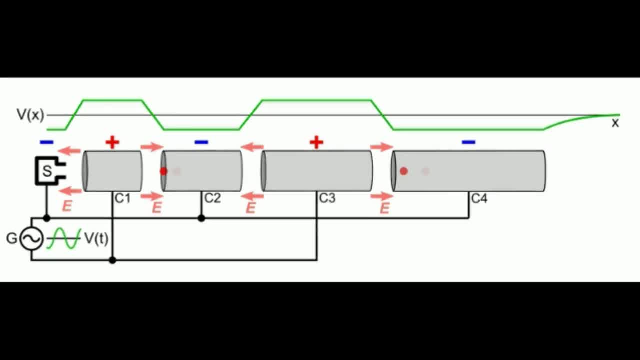 positive electric field and it gets accelerated in the forward direction. now as it enters the second cylinder again, it gets again again the polarity gets reversed and now as it exits the second cylinder again, it experiences acceleration. so every time the charged particle exits a cylinder it experiences a positive electric field and gets accelerated in the process. so during the 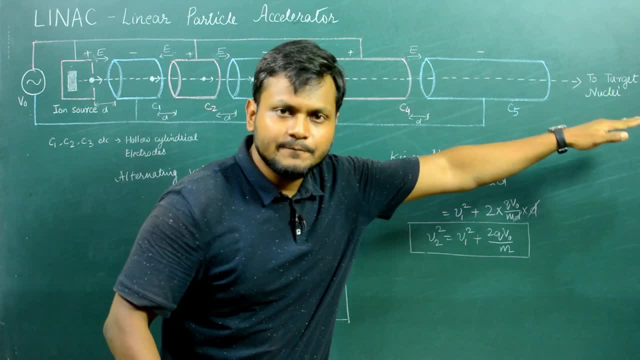 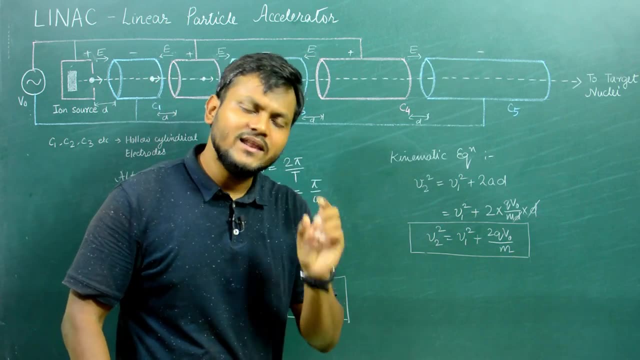 trajectory of motion of this charged particle along a straight line. it experiences these accelerations over and over again and its velocity keeps on increasing rapidly. we can calculate the increase in velocity and the increase in kinetic energy of the charged particle using this simple expression. so let's 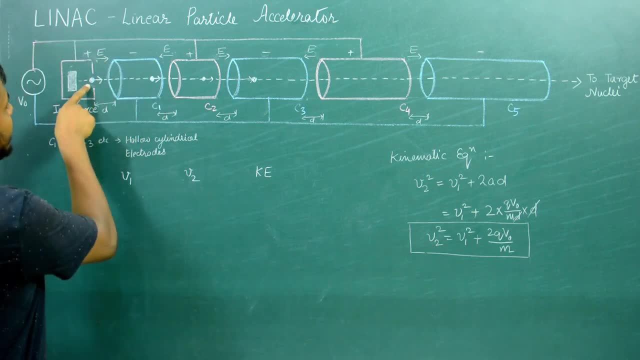 suppose just for the sake of calculation: the moment the charged particle is emitted it basically has zero velocity. let's suppose the charge particle is emitted, it basically has zero velocity. let's suppose for the sake of calculation. so if it has zero velocity as it experiences one acceleration, its velocity is basically increased by this. 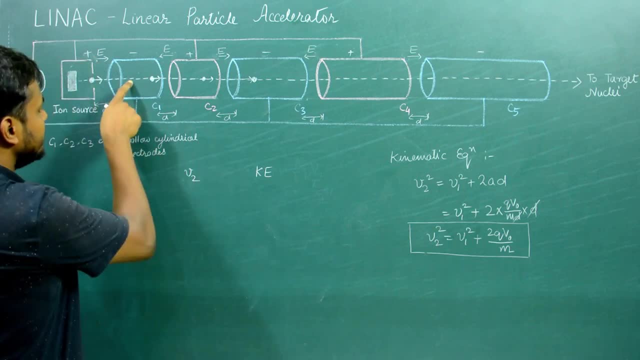 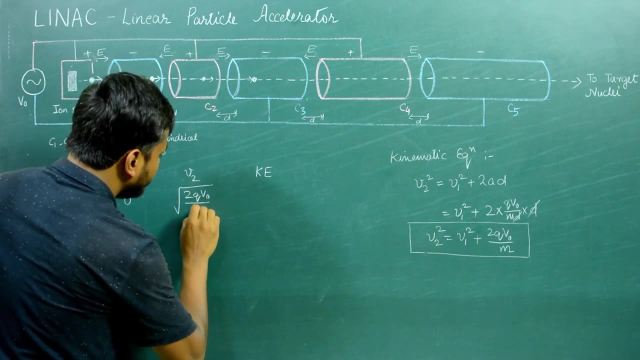 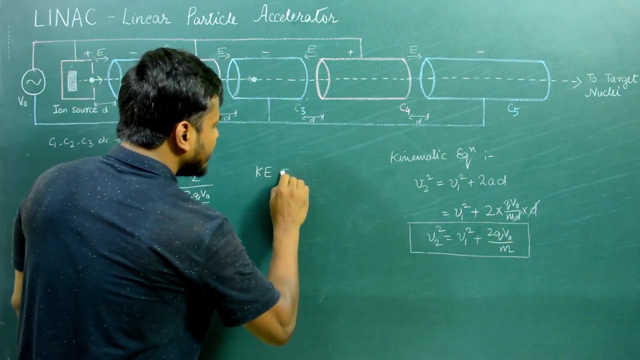 particular amount. so as it enters the next cylinder its velocity basically increases to root over 2 Q V naught upon M. yes, I just put 0 here and V 2 is nothing but root over 2 Q V naught upon M. what is kinetic energy? kinetic energy. 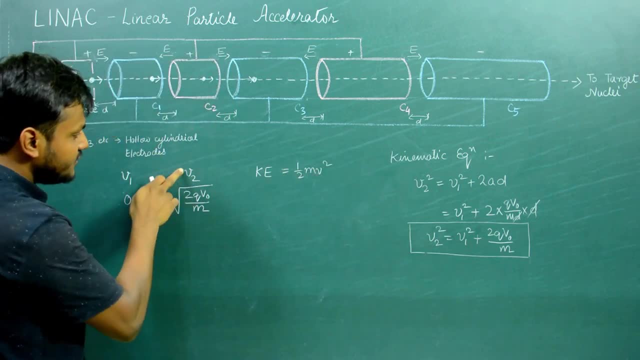 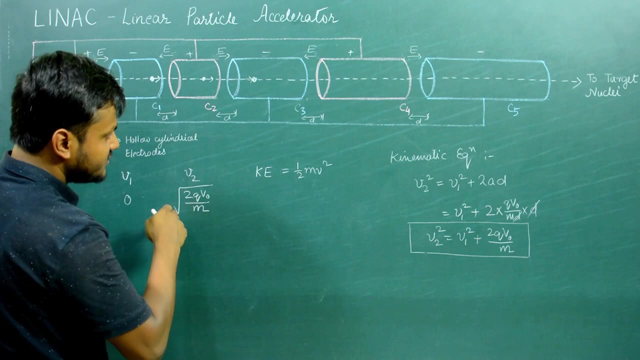 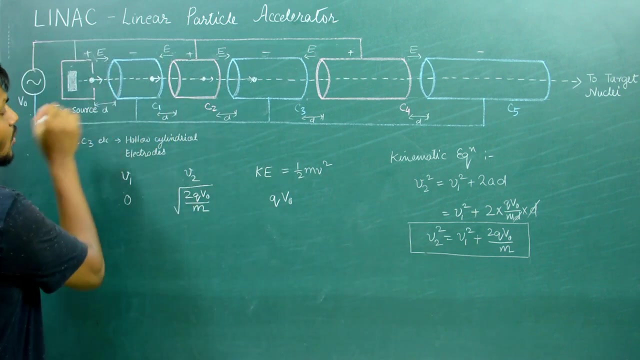 is nothing but half M V square. so the kinetic energy for V 2 now becomes half of M of V square. 2, 1, 2 gets cancelled. V square: the root over gets removed, M&M gets cancelled and the kinetic energy basically becomes Q V directly because of acceleration in one region. now, as the charged particle exits, 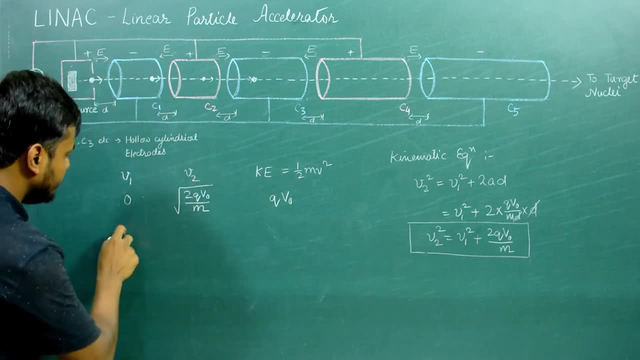 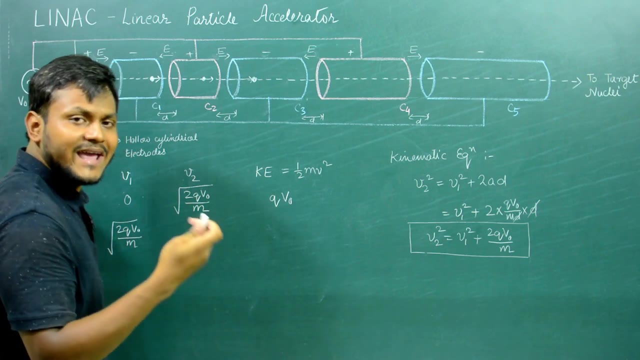 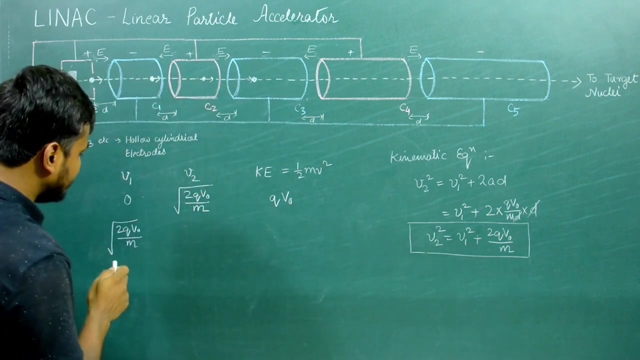 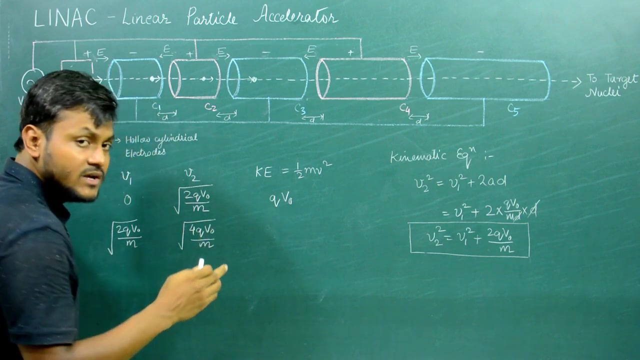 the first cylinder enters the second region. now V 1 is this amount, so the V 1 basically is 2Q V naught upon M. so now is the atoms recombine, so it again gets accelerated by same amount and V to then becomes A, this square plus this, which is basically equal to root over 4 q v naught upon m, so the kinetic. 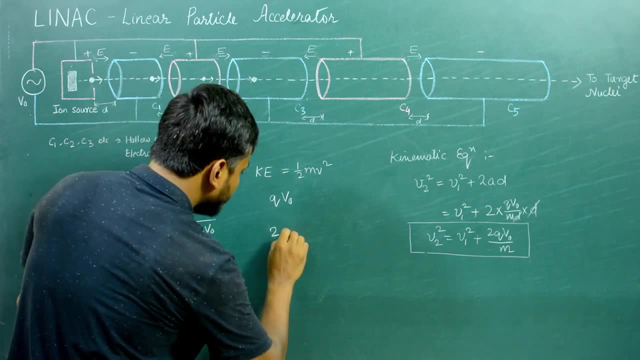 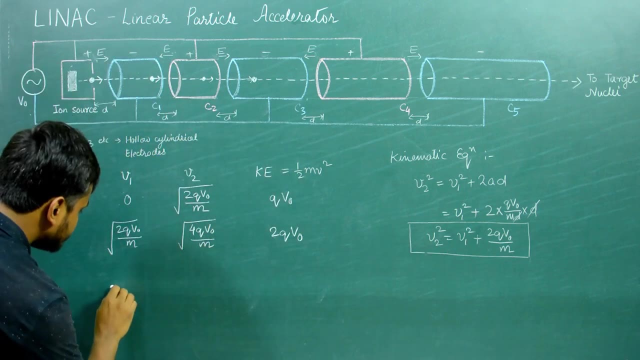 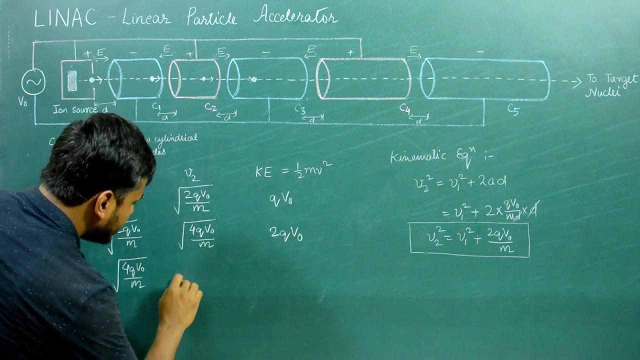 energy- new kinetic energy- basically becomes 2 q v naught again. as a charged particle enters a third region, its velocity of exit is going to be this much and the final velocity because of this is basically going to be equal to 6 q v naught. 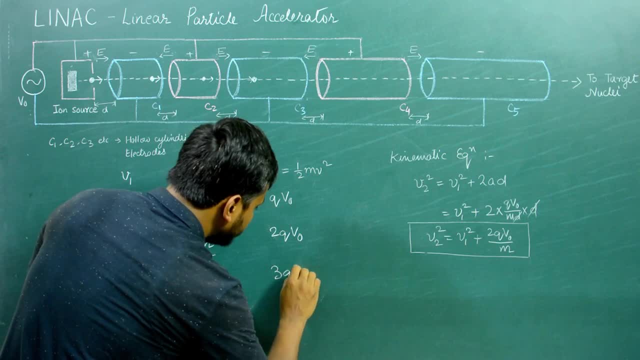 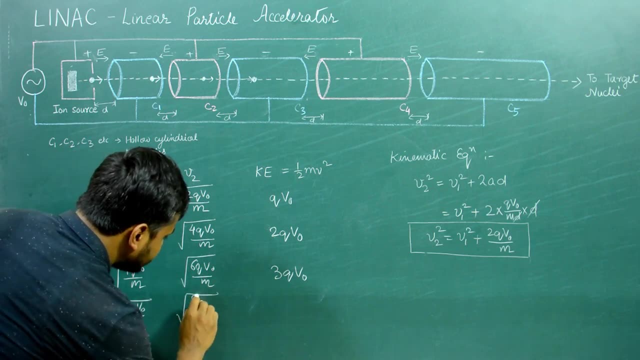 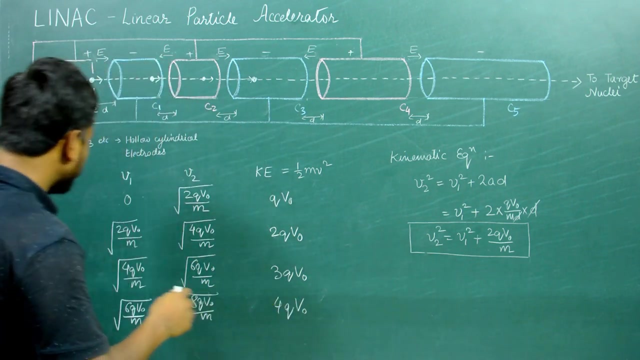 upon m and the kinetic energy is going to be 3 q v naught. and similarly you can have root over 6 q v naught upon m, and then you will have 8 q v naught upon m and the kinetic energy is 4 q v naught. so, as you can see here, with every next region, 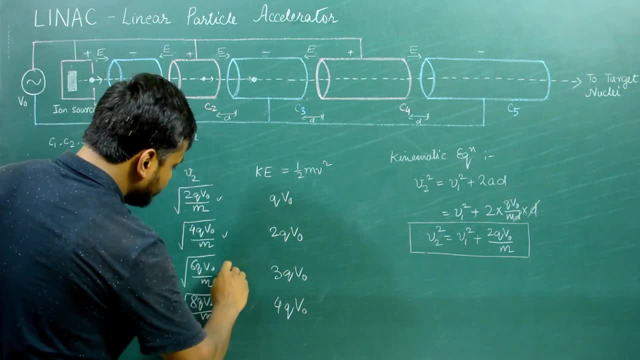 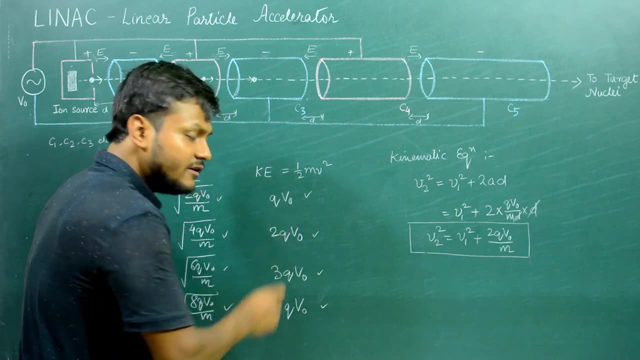 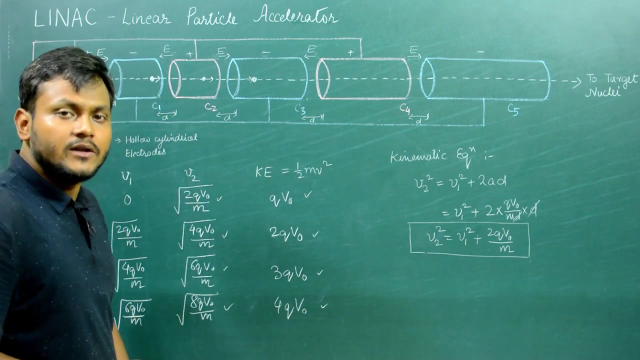 the velocity of the charged particle keeps on increasing and the kinetic energy of the charged particle keeps on increasing. so even though the potential difference v naught itself is maybe not very, very high, if we can make the charged particle go in this particular manner over and over and over again, we can increase the kinetic energy to very, very high. 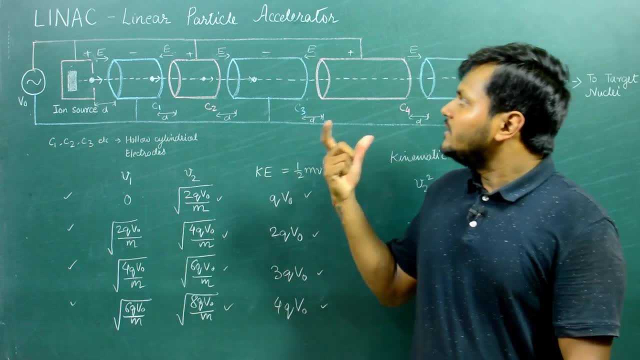 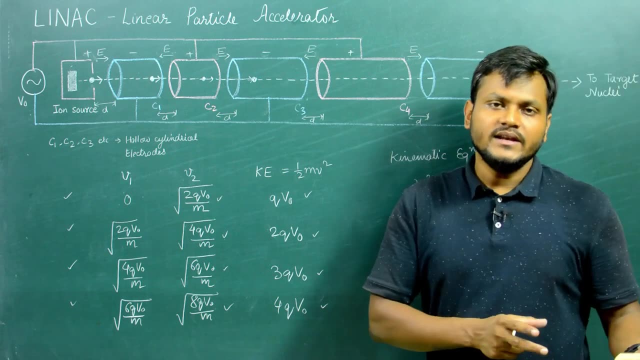 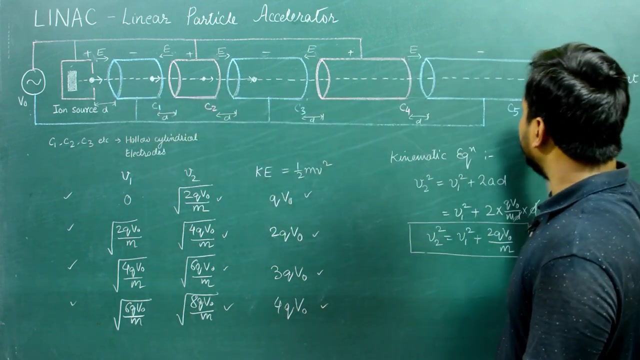 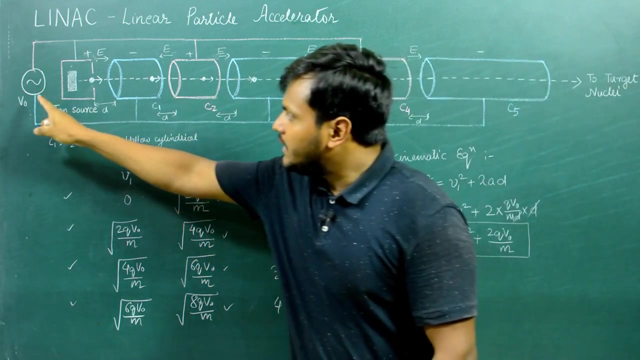 values. in fact, the linear particle accelerator can accelerate charged particles to extremely high energy, So the kinetic energy is even greater than the Van de Graaff generator, for example. however, there is a limitation to this kind of a setup, because the charged particle is getting accelerated in one particular direction as its velocity keeps on increasing. now, because the time period